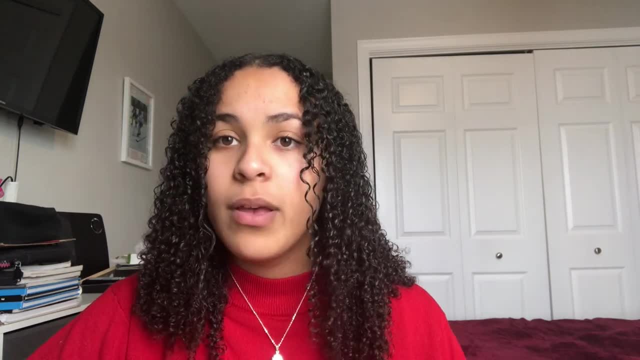 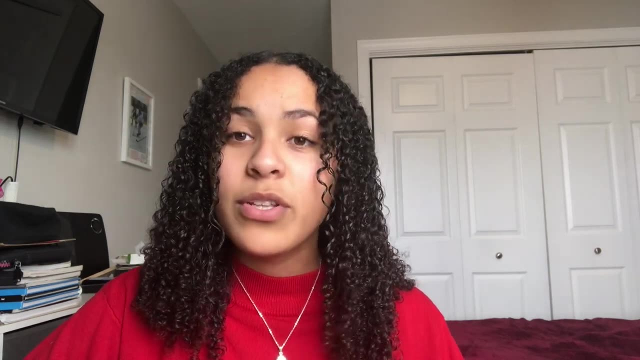 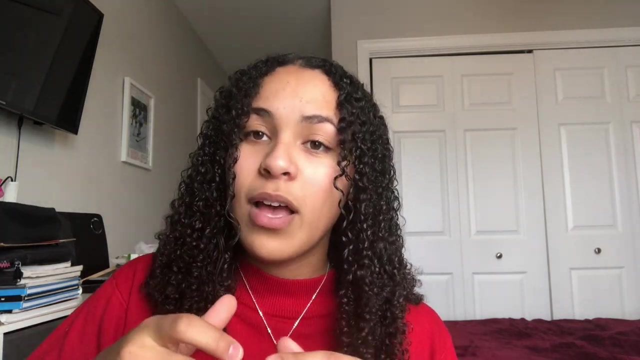 And I'm going to show you kind of some ways to work through it. I'm going to switch to my iPad view just to work through some practice questions that I got from armytestcom And I'm also going to print out the shapes from those questions and I'm going to show you how they actually fold up. 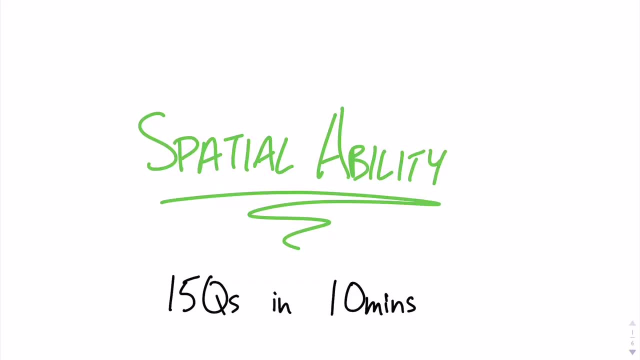 So now we're on the iPad looking at the spatial ability section. Just to remind you, there's 15 questions which need to be completed in 10 minutes, So that means that you have to do more than one question per minute, or in other words, you have less than one minute per question. 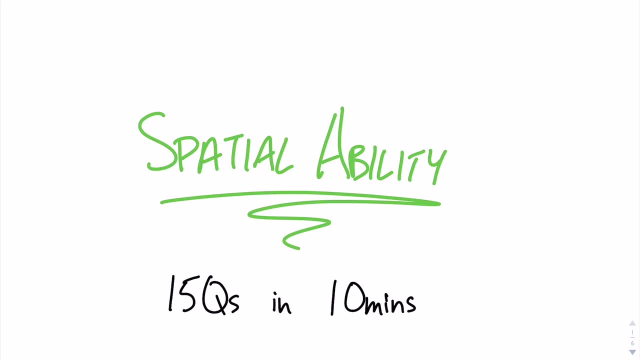 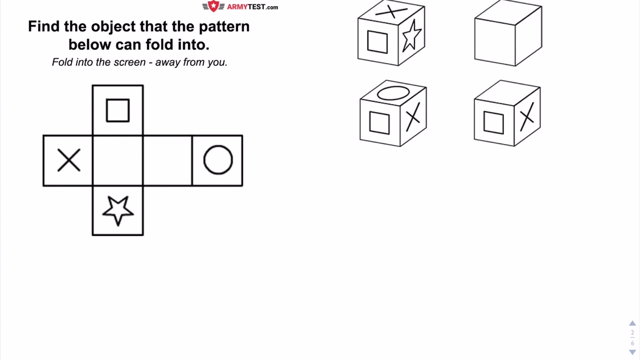 Now, this makes this section quite challenging, because you need to fold and unfold 3D objects in your mind In order to answer the questions. So to explain what I mean by that, let's look at the first question here, Which says: find the object that the pattern below can fold into. 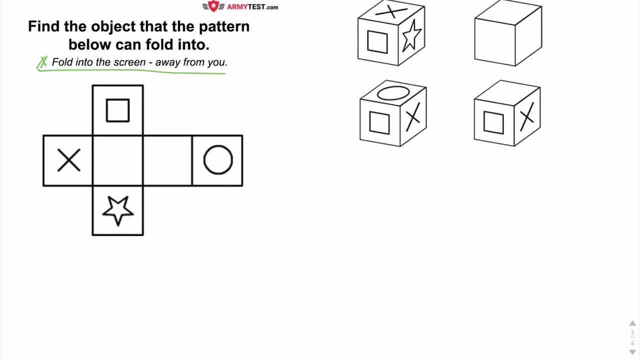 Fold into the screen away from you. Okay, So basically what that means is that you're going to fold everything backwards rather than folding everything towards you. So just to tell you what I mean, or just to explain what I mean a bit better: 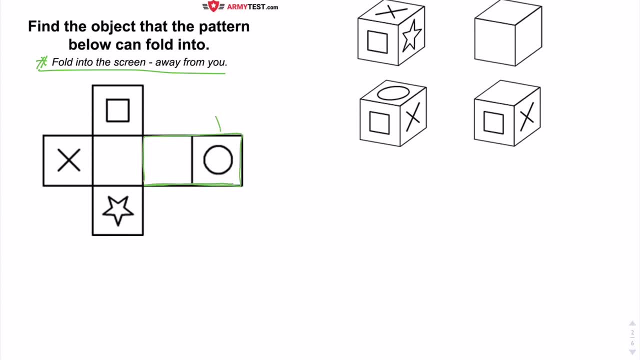 If you were to look at this section here, if we were folding this away from you, then it would become something like this: right Now, if we were to fold it towards you, which is incorrect, it would become something like this: right. 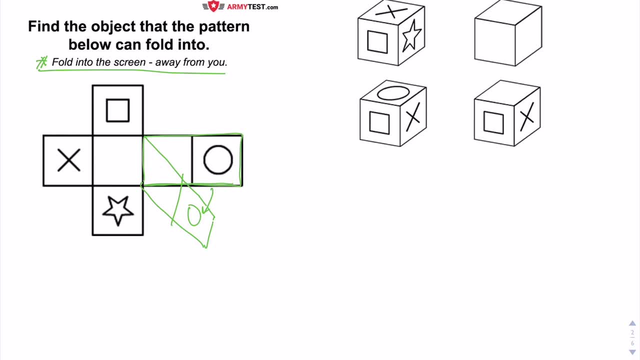 That would be like poking out of the screen towards you. Alright, so just keep that in mind. Now, with these types of questions, the first thing I like to do is eliminate any obviously incorrect options. So from looking at this, this option here kind of sticks out to me. 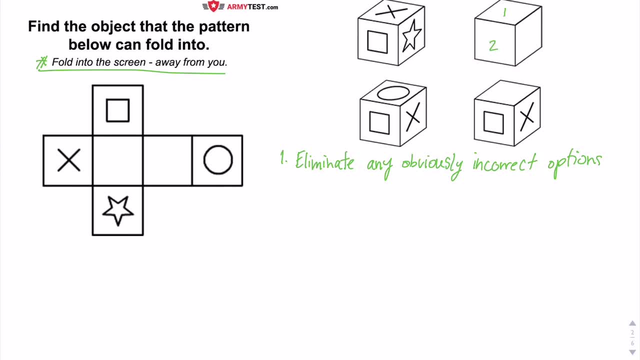 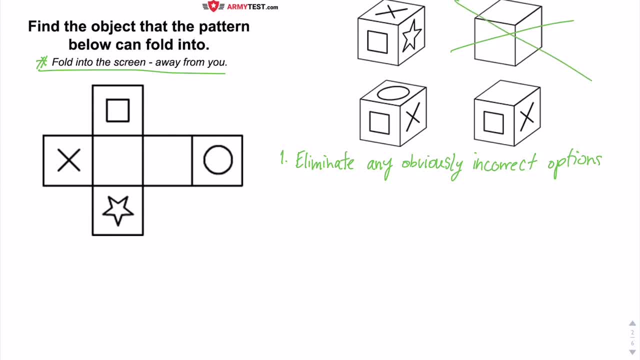 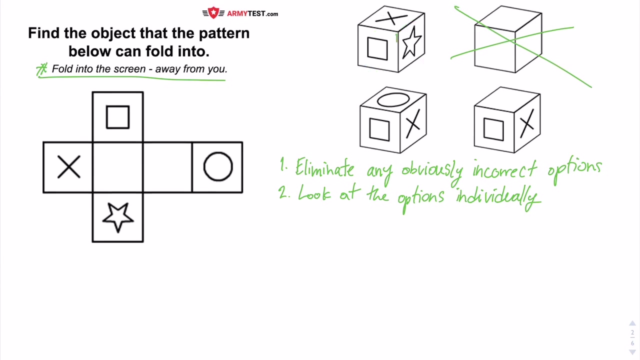 Right, But our map or our projection only has one face, correct. okay, now moving on, we can now look at other options. look at the options individually. so now we're going to look at this first one here, so we can look at how these two shapes are related, and that is through this connection here. 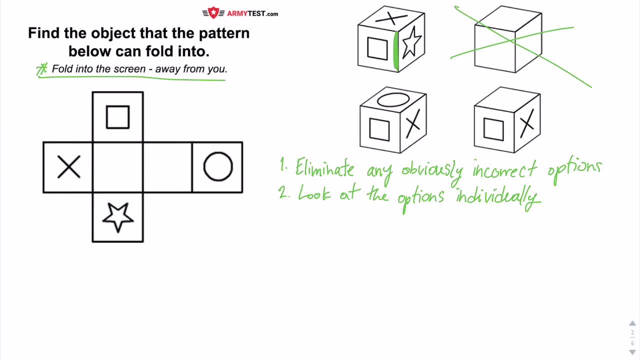 so they're connected by an edge, and I'm looking at these two shapes because that's what makes this option different from these two options, because these two options have the same, you know, square X, square X, or this one has square star. so that's why I'm using this relationship to try and 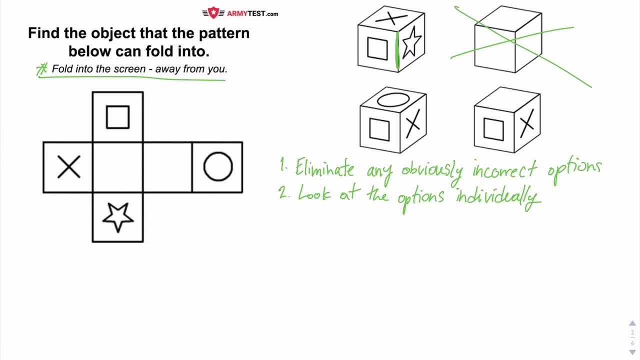 see if that's correct or incorrect. alright, so if we look at our map or projection here, we can see that if we look at where the square is and where the star is, these two do not share an edge. share an edge, okay. so I'm just going to illustrate this by simply trying to draw this for you. so let's say: 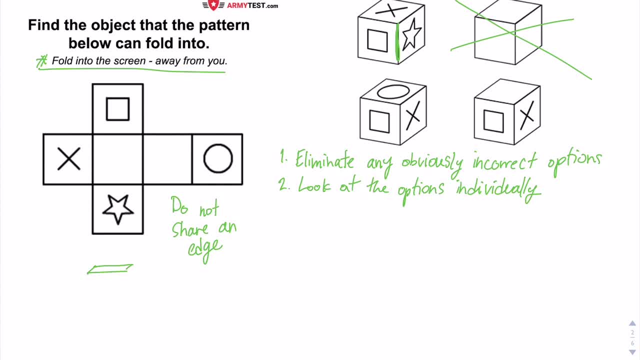 that this is the bottom, is at the bottom and blank one, that top face, and on the side here you would have the square and on the other side you would have the star. okay, so there's a big space here, right? clearly these two cannot share an edge, unless it was like a triangle type of thing. right, because then they would share this. 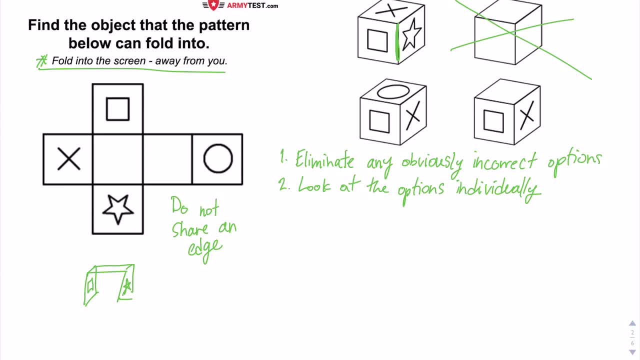 edge, but that's not what's happening. right, they need to be connected by a whole another face here. so therefore, this is not the right answer. okay, so now we can look at these two options here and what differentiates one from another? well, it's this top face. this one has a circle and this one is blank. so let's figure out which. 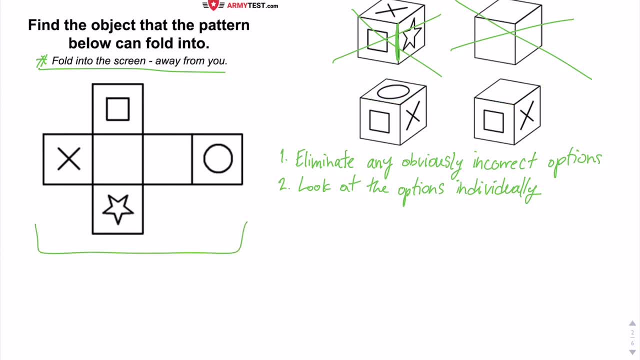 one of those is correct by looking at the given projection. now, if we were to fold this up so that we had a square and an x beside each other, that would mean we have to fold it along this edge, right? so let me just do that here. so we have the square here and then the X, and then this. 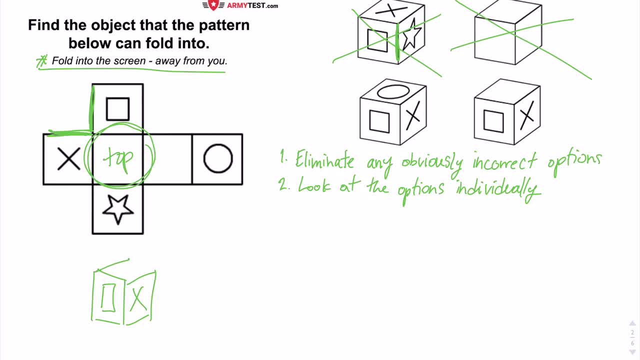 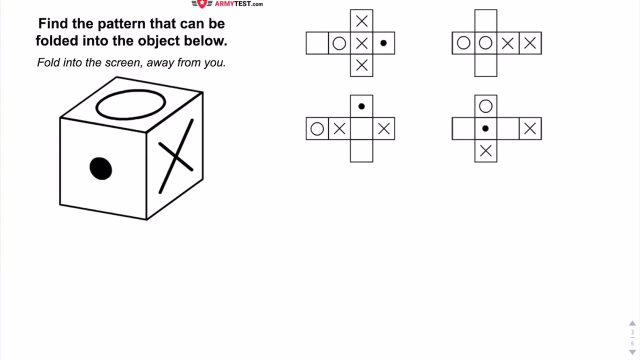 would be the top face. okay, so the top face would be blank, all right. so out of these two options, this one clearly has the blank top face and therefore it is the right answer. all right, so this one is incorrect. so moving on to the second question. here, this one says: find the pattern that can be folded into the 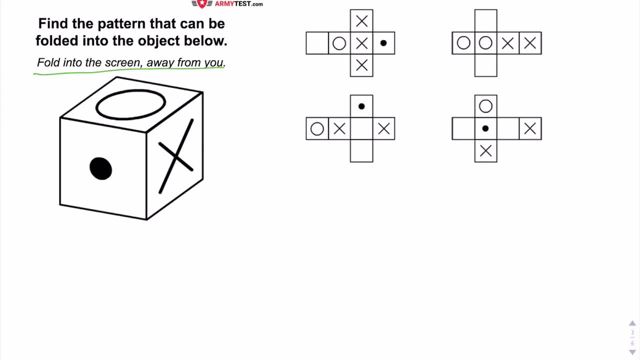 object below fold into the screen away from you. so same hint as before, and this is kind of the reverse of what we just did. so again, you want to start by eliminating, or eliminate any obvious options, obviously incorrect options. so how are we going to identify these incorrect? 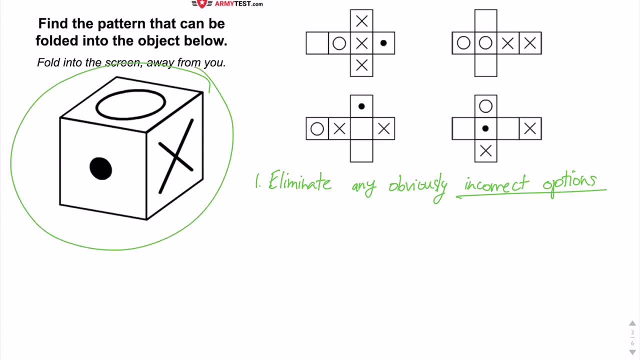 options. well, we can look at what is given to us here. so we are given a cube that has a circle dot and X on its faces. therefore, our projection must have a circle dot and an X, right, let me fix that so that can be our first check. so let's go through and see to make sure that all 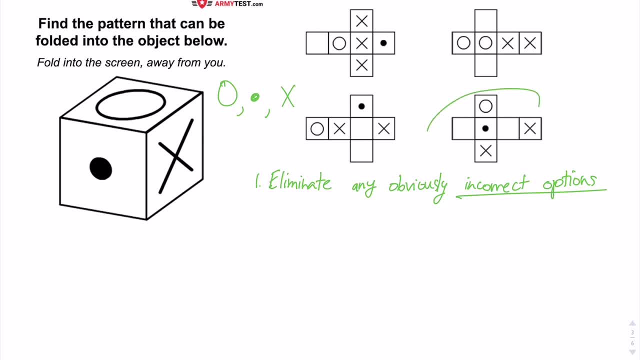 of them have those three components. so looking at this one here, it does in fact have an X, it has a circle and it has a dot. so that's great. next one has an X, has a circle, it has a dot. okay, next one circle, dot X, next one circle, but no dot. 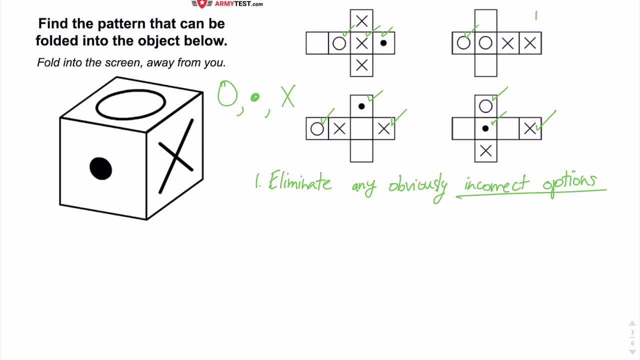 therefore, this should be an x in a horizontal order for the same thing. let's, this one can be eliminated right away. right? So that first step got us down to three options, which is great. So now what we want to do is look at each option. So, out of the remaining, 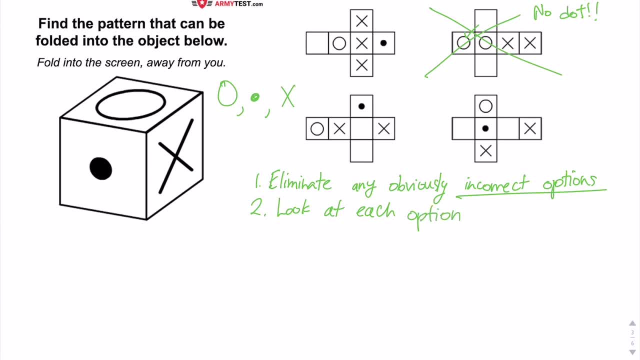 three options. let's look at each of them Now. one trick that I would use for this question is to identify that we should be folding each of the projections around the dot in order to receive this orientation after folding. So to show you what I mean, let's start with. 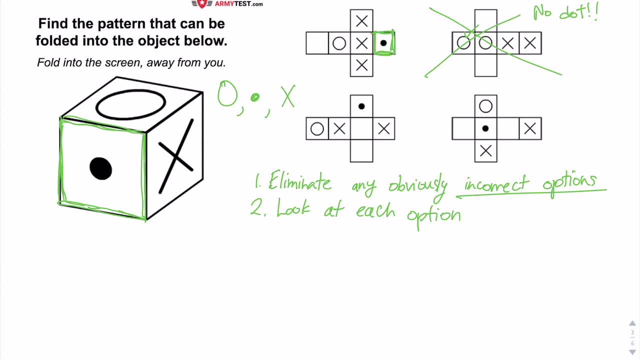 this one here and we're going to fold it around this dot. So I'm going to call this A right A here. I'm going to start with that face, So I'm going to put the dot right here and then I'm going to fold the other things around it. So this would be the top. 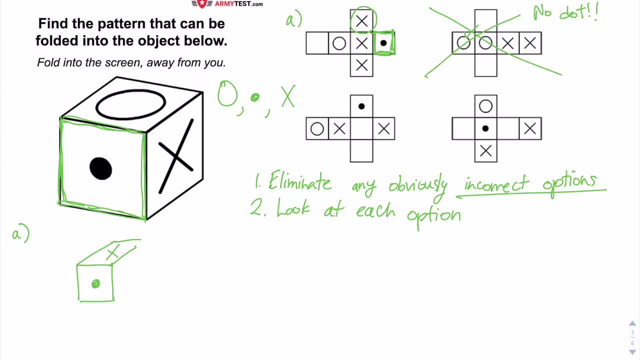 face here. This would be the left-hand side face, which you can't see. so I'm just going to draw like that. This would be the bottom. So again, right there, You can't see it. Then this would be the back. So this would be over here And the right-hand side would be blank. So I'm 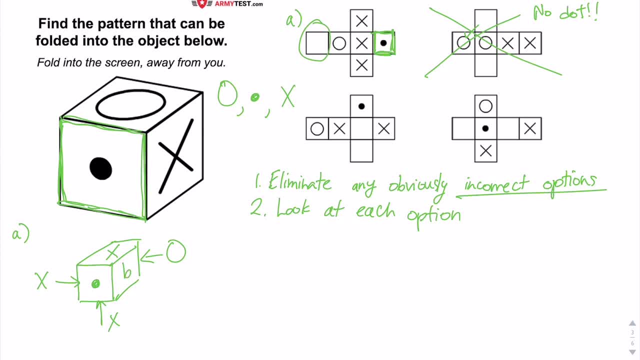 going to write B for blank. I'm just going to say B equals blank. Okay, So clearly this option is incorrect, right? Because when you compare these two, the correct answer has a circle up here and an X right here, But the answer we came up with does. 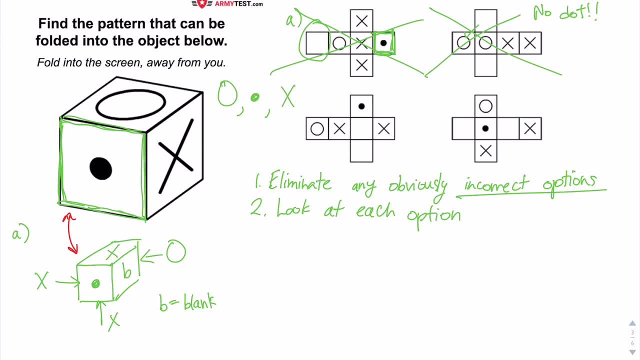 not All right. So, moving on to the next one, I'm going to call this one B B And again, we're going to fold it around this dot. So this would be the bottom. So I'm going to fold it around this dot. So, starting with that dot there, Fix this side. So this is. 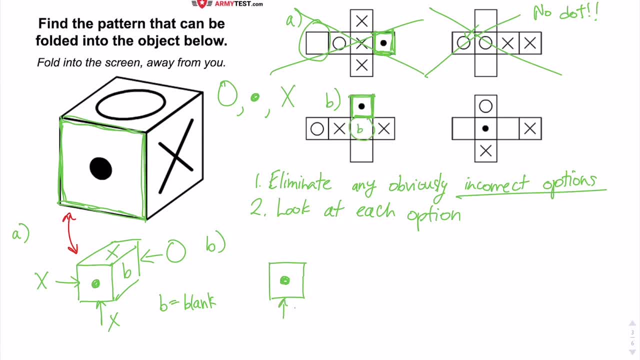 going to be the bottom B for blank. This will be the right face, So this is going to be an X there, And then this will be the back face. Okay, This one is going to be the left face. So over here And then the circle. here is 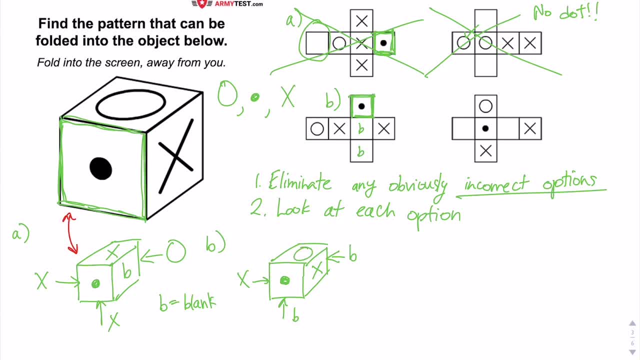 going to be on the top. Boom. Look at that. Now we can compare these two And it's correct, right, So you have the X, the circle and the dot, Therefore B as I've called it. 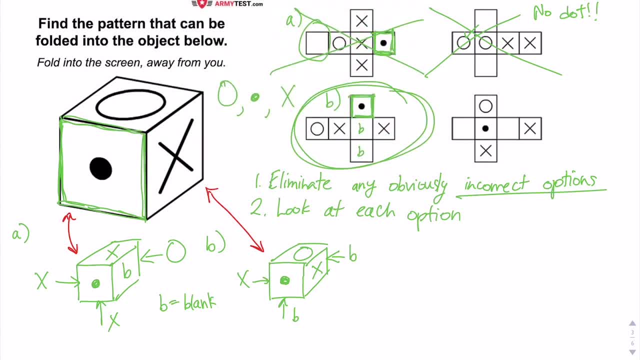 is the correct answer. So we can circle that. Just practice sake, let's do the last one, which I will call C. So again, we're going to start with this dot and we're going to fold around it. So I'm going to start by drawing. 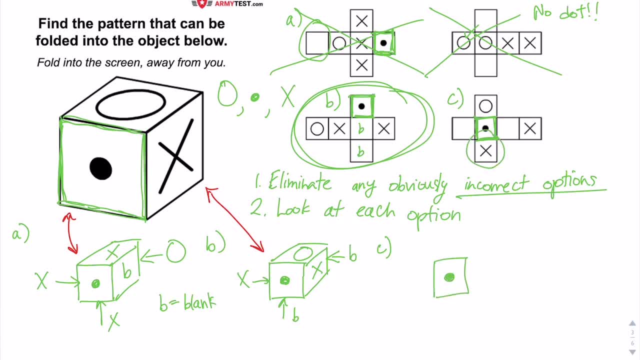 that dot. So this will be the bottom right here. X, That face. This will be the right hand side B for blank. This X will be at the back. I'm going to draw like that. This blank will be the left which will be here, And then this X will be at the bottom. So 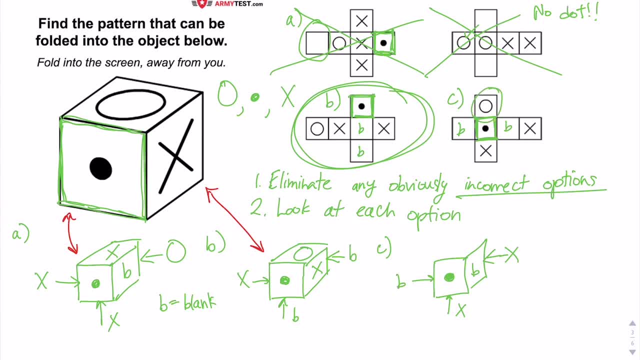 B for blank, And this circle will be on the top like that Right Now comparing them. so, comparing the given box to the one that we came up with, we can see that in order for this to be the correct answer, we would need to have an X here, which we don't. So 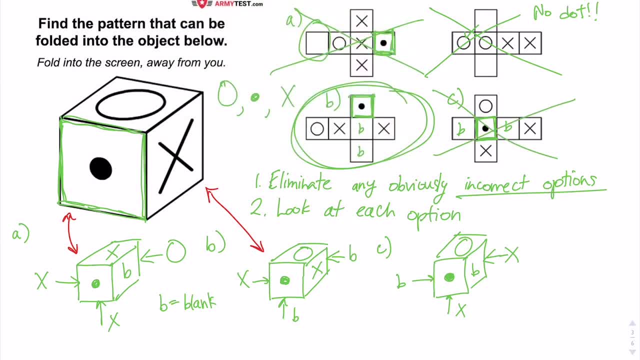 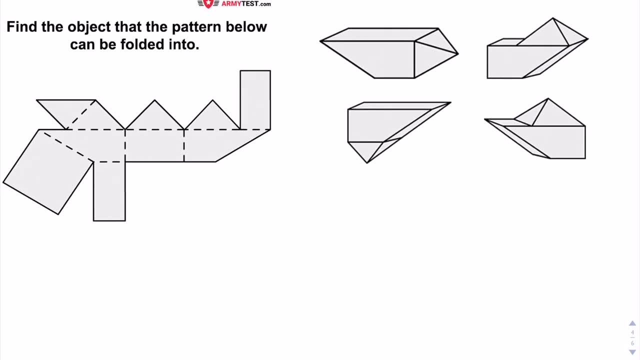 therefore, this answer is also incorrect. Okay, So moving on to our last question here, Which says: find the object that the pattern below can be folded into. Now, looking at this might be a little intimidating, but this is a great example of a CFAT question, because 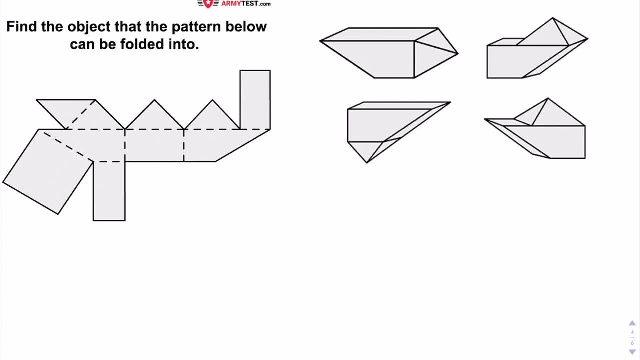 they are not all boxes that you're folding. Okay, So this is a funky shape, but in fact you may get something like this, So let's just go through this. So what we were doing before was we were trying to eliminate one right off the bat, So we were trying to look. 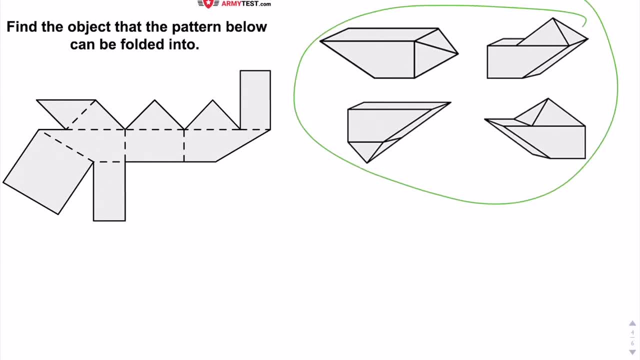 at these and say which one doesn't belong here. It's not obvious. It's not obvious. So we're going to move on to step two, which is to look at each of these options, And we're just going to see what similarities and differences. 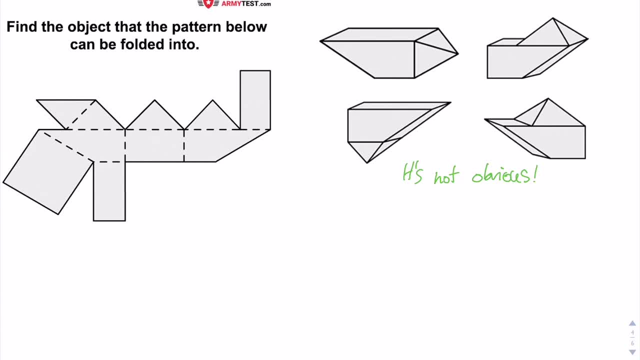 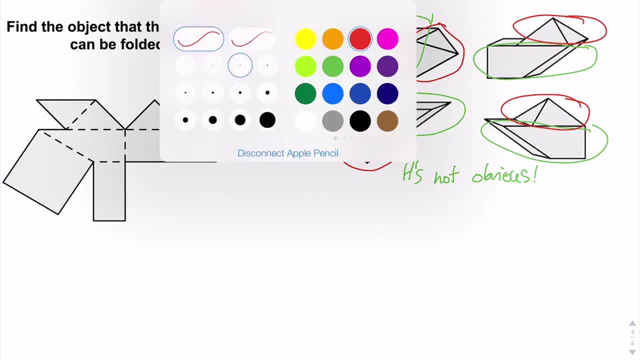 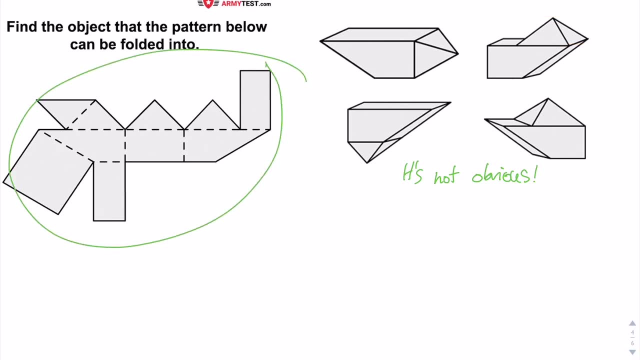 per se. So, with that in mind, I'm just going to erase these, And let's start over here and try and fold it up, just to see which one will match. Okay, So I'm going to start with this section right here and fold it up. 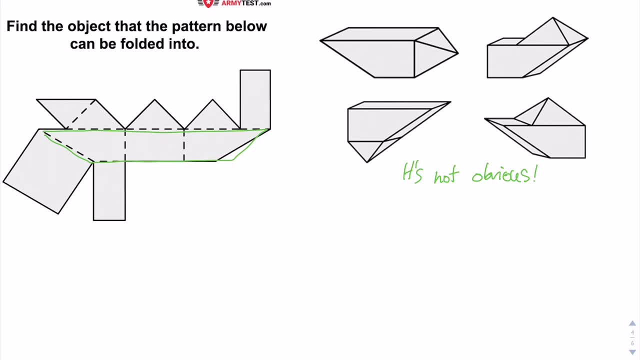 Just because I'm thinking of that as, like, the body, and then this would be the top attachments and these would be the bottom attachments. So that's just how I'm splitting this up to make it a bit simpler. So if I were to fold this section up, I'm going to get something. 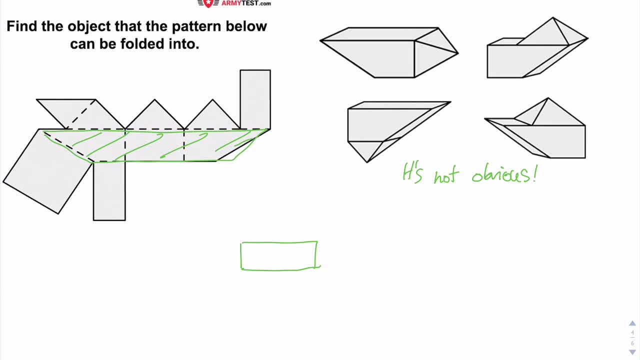 that looks like. try and draw this here, something that looks like that. Okay, Now I'm going to look at these triangles which are on the top. Alright, So just by looking at this center piece. the first triangle is connected by this face, So that is right here, Just so. 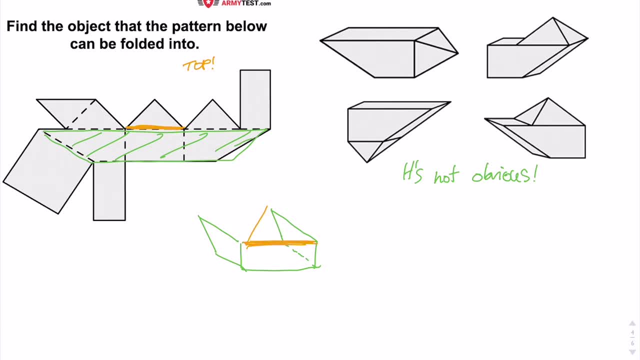 you can follow what I'm doing here. So I'm going to draw a triangle on here. Okay, This is going to be hard to see, but I'm going to try my best to explain it Now. this next triangle attached by this edge, which is this edge here, so you can't really see that. but 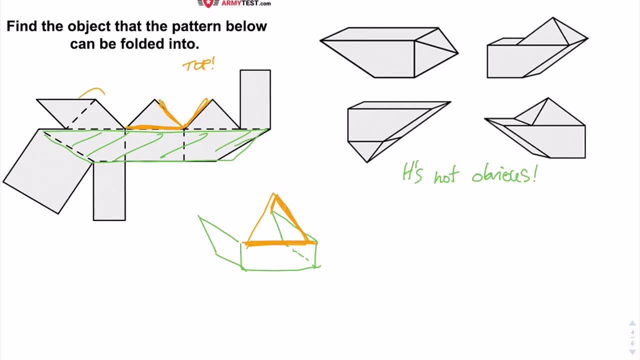 I'm just gonna draw the triangle. this triangle it's gonna be attached via these edges, so that would be one edge which is here. it's gonna be something like this and it's also attached here, which you can see is right there. so that's in the right place. okay, I'm actually gonna extend this part a bit. 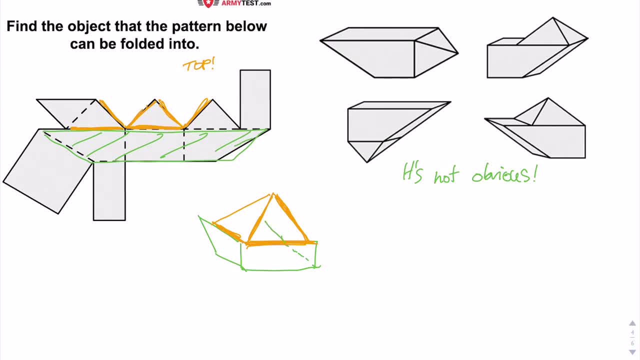 you'll see why in a second. but I don't want this to connect to the whole length of this shape, because it doesn't connect to the whole length, so I'm just gonna attach it to this part as a triangle, and then this triangle here is attached by this face, so it will just enclose the shape. so this is our. 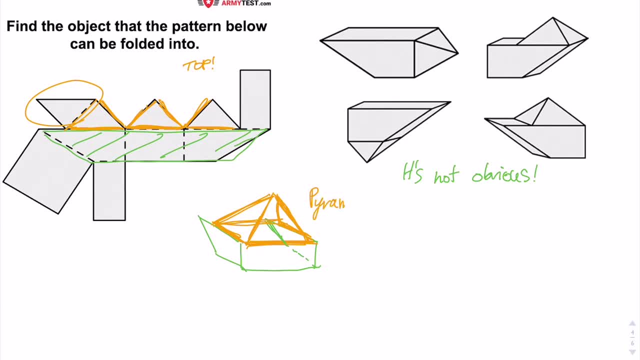 pyramid. okay, now I'm gonna look at this rectangular piece right here which is attached to this piece. so that's why I need to extend that green piece, because this blue piece will attach to the end of it and go all the way across. like that, it's a rectangle. next we can look at this purple shape, purple rectangle- and 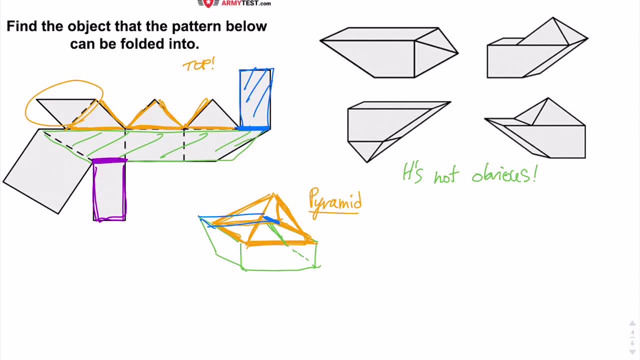 that's just attached to the bottom horizontal parts of this piece which is right here and it's gonna fold up across here. so that's gonna be the bottom. and now you can look at this square here which is attached to this slanted piece. so this is the slanted piece and it's gonna lay right off your face. so that's. 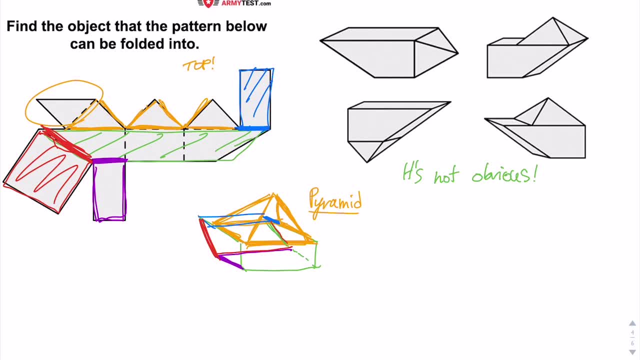 right across here. Now, this is probably very hard for you to see, so what I'm going to do is I'm going to kind of rotate the image, which will give you a better sense. I'm going to rotate it that way, so I'm going to draw this slanted piece here. so I can't draw this straight, apparently. 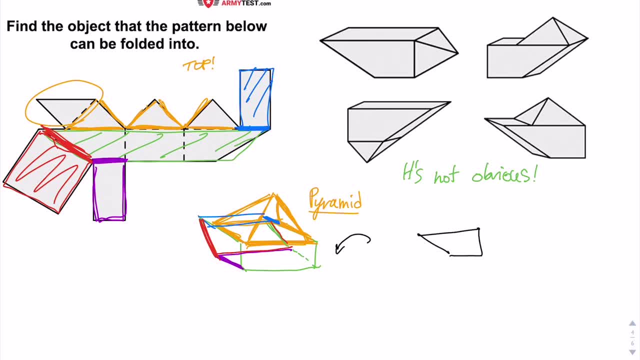 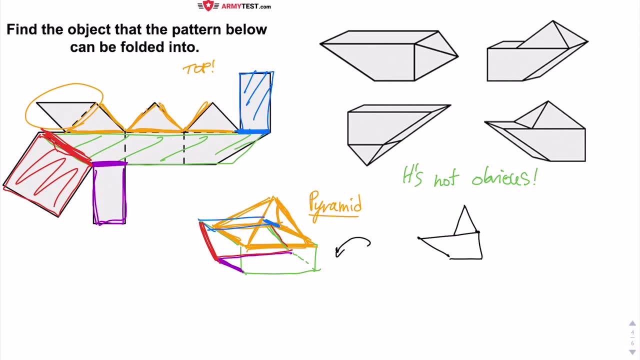 and then you're going to have the triangular pyramid up here. I'm going to try and draw this in 3D, actually like this, like that, something like that. you get the idea. So just to highlight what I'm saying is, the triangular piece is here, then we have the 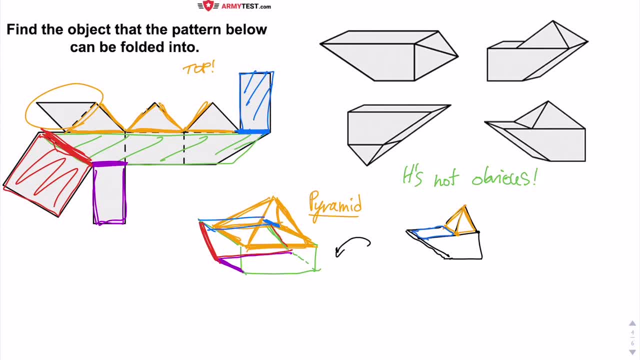 you have the blue piece, which is this, we have the green piece, which is this, and you can also see the front piece from this view, which is right here. All right, so what does this look like? Well, it looks like this. So this is actually the correct answer, but I want to point out why the 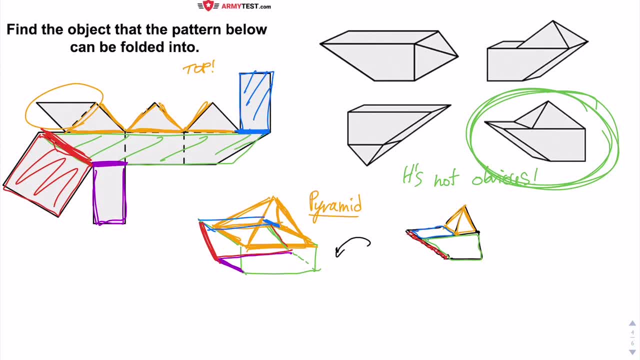 other ones are incorrect. Okay, So if you look at this one, the triangular piece, or the pyramid, is up here right, but it's attached to this edge. so if that were true, this triangular shape would have to be pulled to the front right and it would have to be. 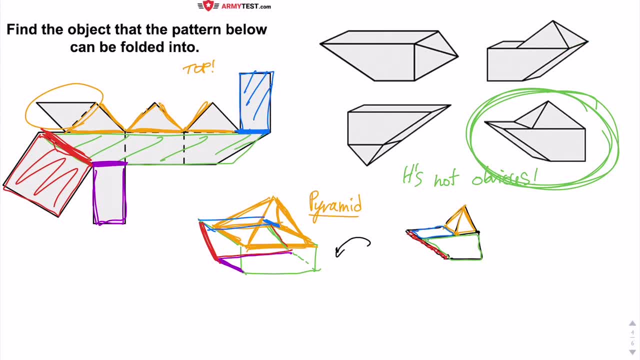 attached to the slanted edge, which it's not. so this would be correct if you pulled this back to this edge here, But right now it's incorrect. For this one. the pyramid is attached to the rectangular piece, Which means that it would have had to have been attached to this rectangle here. 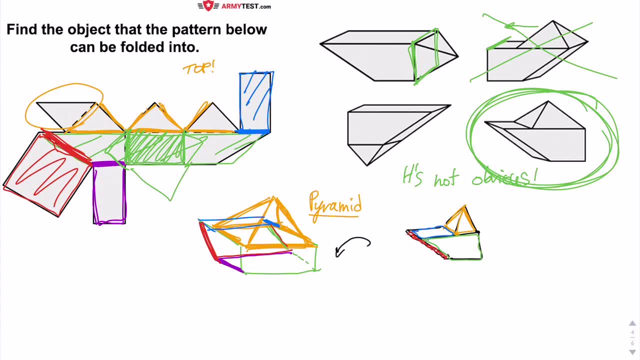 On all four sides, Like that, Which it's not. Sorry. that's really hard to see, But that's why that one's incorrect, And this one shows the pyramid at the bottom, Which means that it would have had to have been attached to these pieces here. 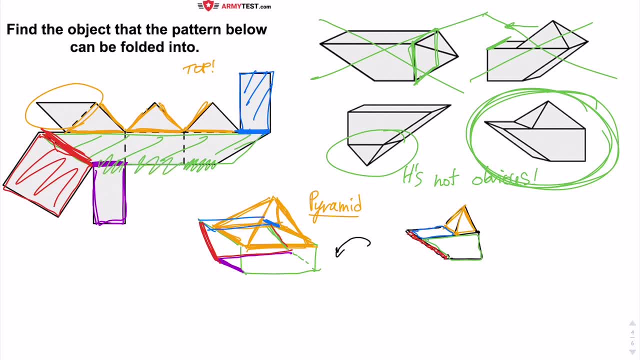 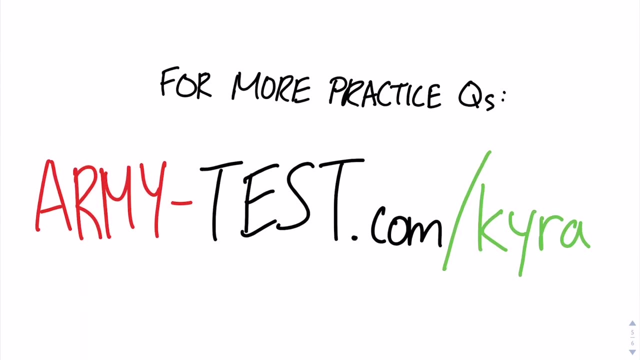 And here and here In order to make that work. So that is also incorrect. So I hope that helped you guys understand how to do these problems. If you need more practice with these questions, as I've mentioned before, there's tons of practice questions at armytestcom. 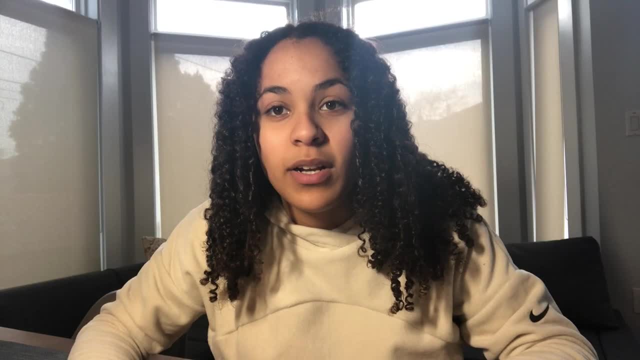 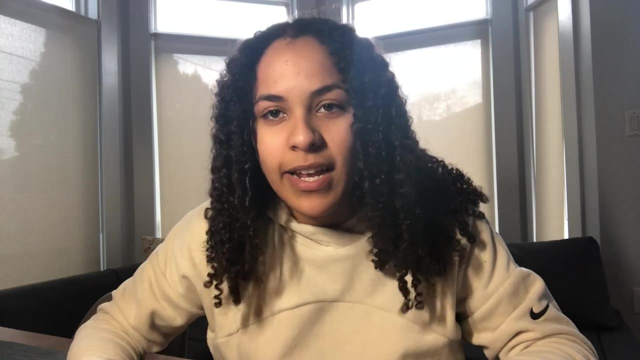 So feel free to check it out and thanks for watching. Okay, so I wanted a better way to show you guys. You know how to actually visualize these things And although you can't do this on a test, I thought I'd just put it in anyways. 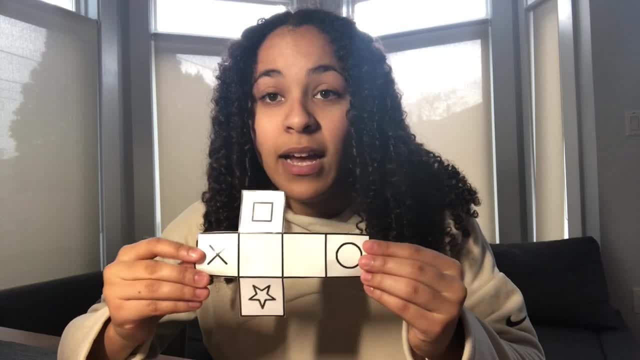 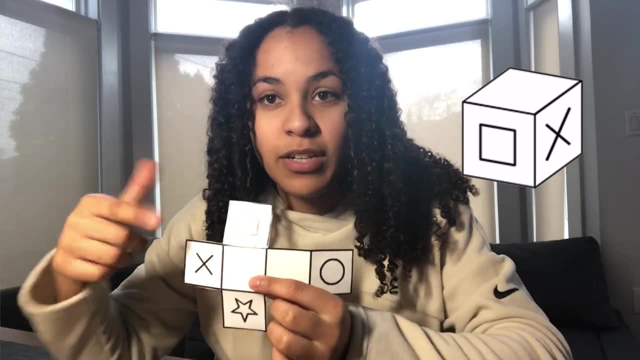 So the first one that we had was this: Right, And if you remember, the answer to this question number one was this: Now, what I'm gonna do is I'm just gonna fold it up and show you that you do get the right answer. 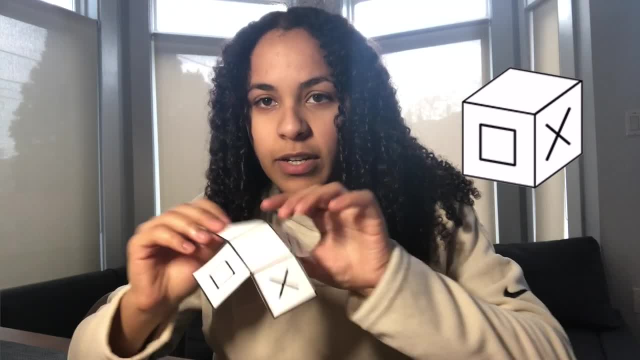 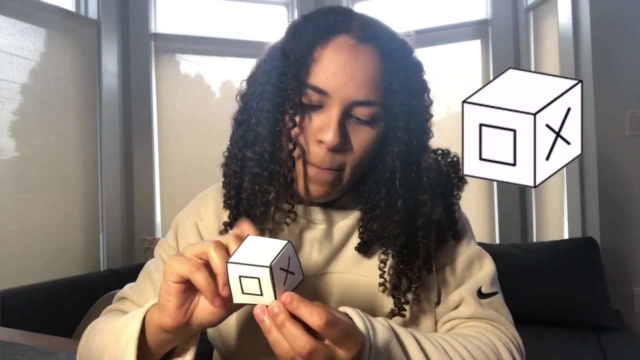 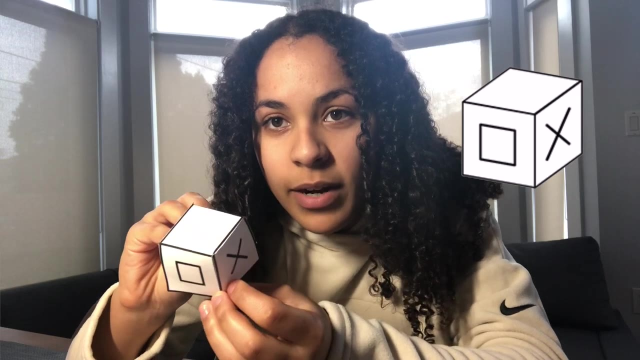 Alright, So I'm gonna turn it so that you can see that the X and the square align together like so: Boop, boop, boop, And you really do get that blank face on the top. So it's X, square, blank face, which was the answer. 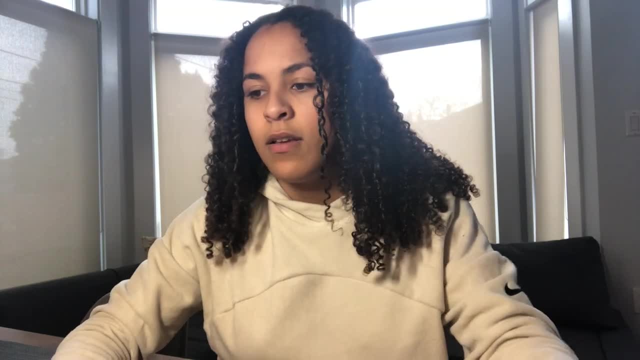 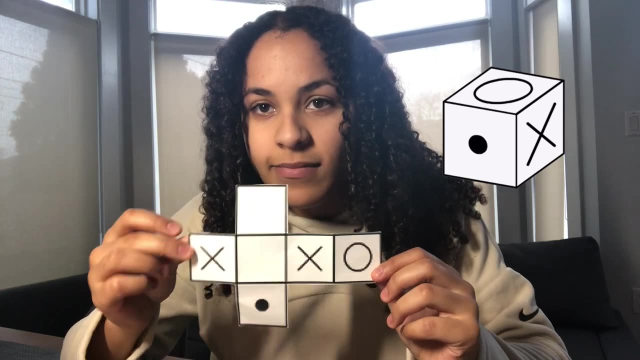 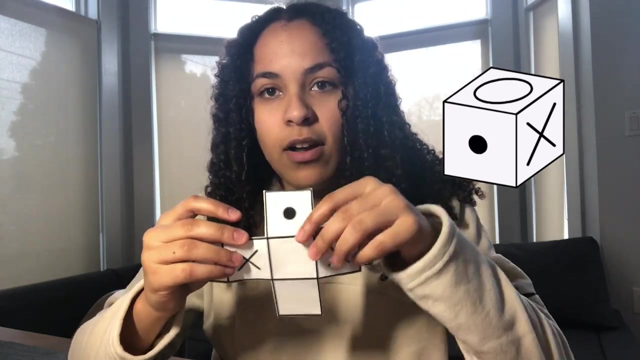 Okay. The second one gave you a cube. that was this, And then this was the right answer. Okay, So I'm just gonna fold this up and show you how this is the right answer, Starting with- Let me turn around, Starting with- this dot. 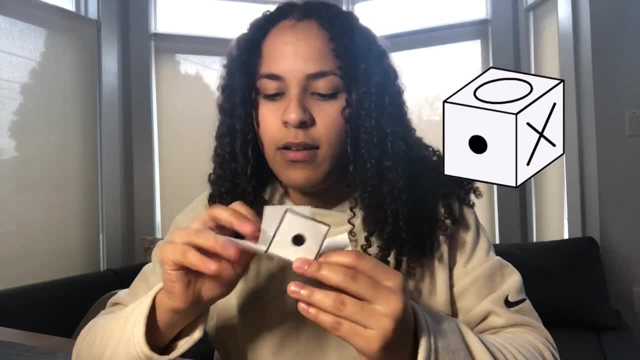 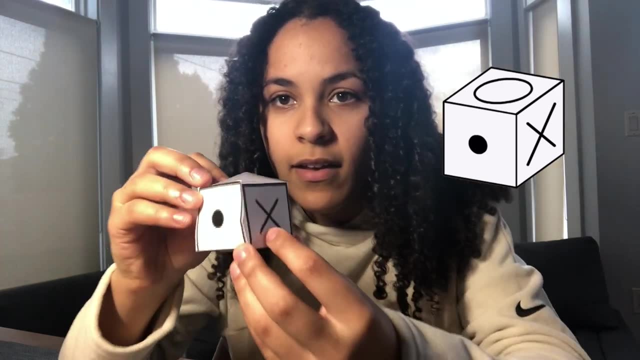 So I'm gonna make this the face, So I'm gonna fold up the back, Fold, fold, fold, Fold, fold. And what do we get? We get a dot, an X and a circle on the top Right. 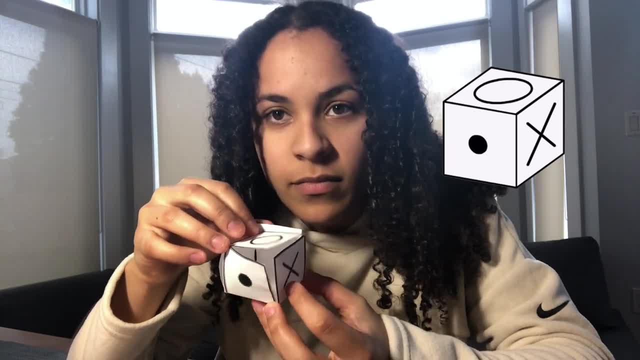 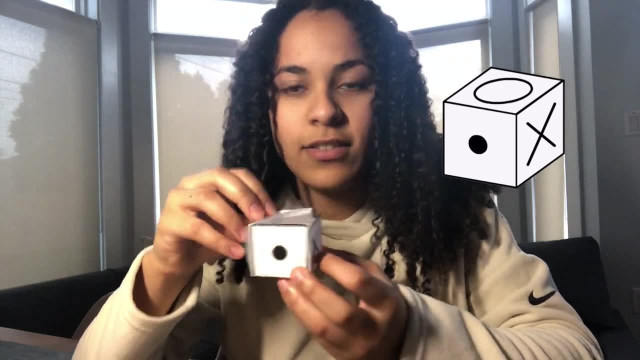 And that was the answer. So this is pretty low quality, but I think you can see what I'm saying. I have the dot, the X and the circle. Now, the last one that was hard to visualize was this shape And if you remember the end, 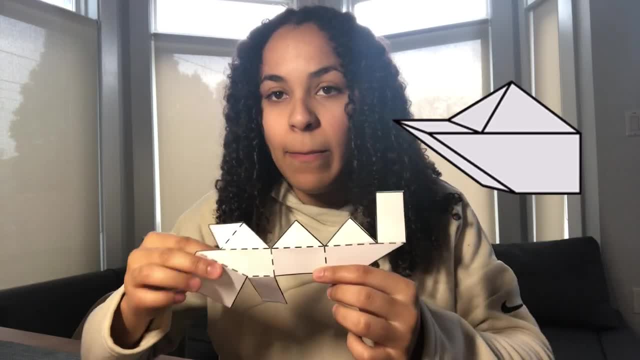 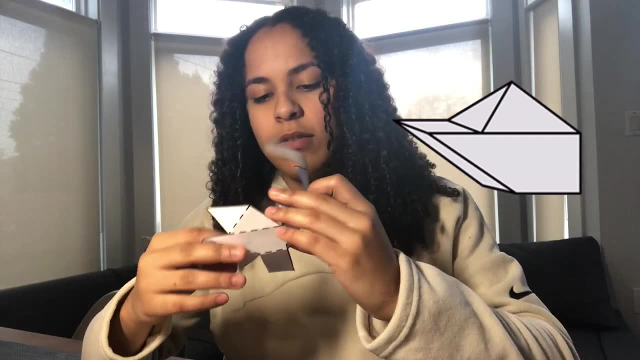 If you remember, the answer was this. So I'm just gonna fold this up, Try my best to fold it up and show you that we do in fact get that shape. So I'm just gonna fold this around. Fold the back up. 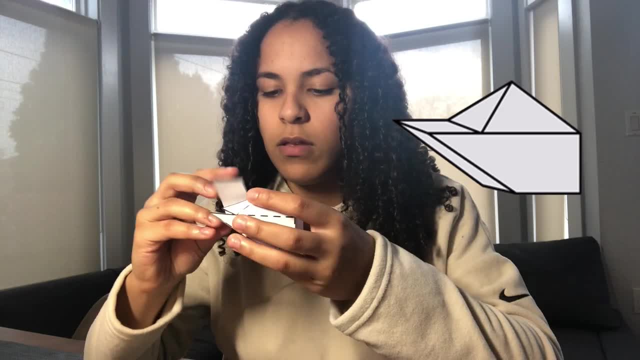 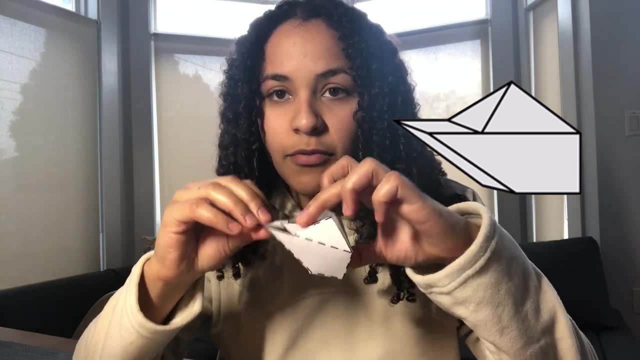 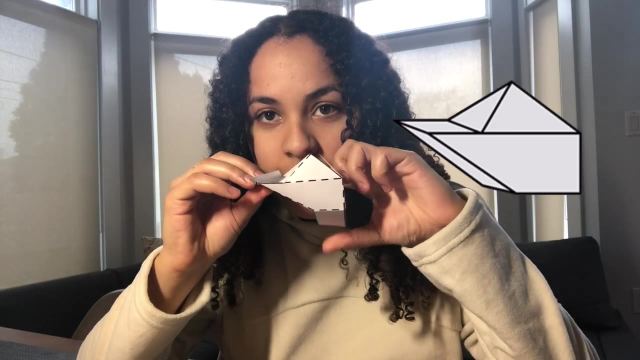 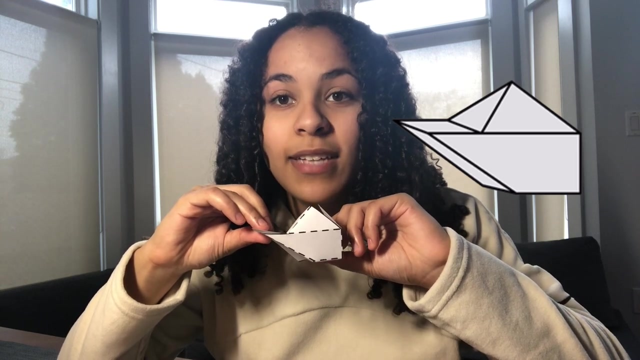 Fold the base up. Okay, Push that down, All right. So this is pretty rough, But You can see that you do in fact get that shape, The shape where that triangular square-based pyramid was at the back, at this edge. 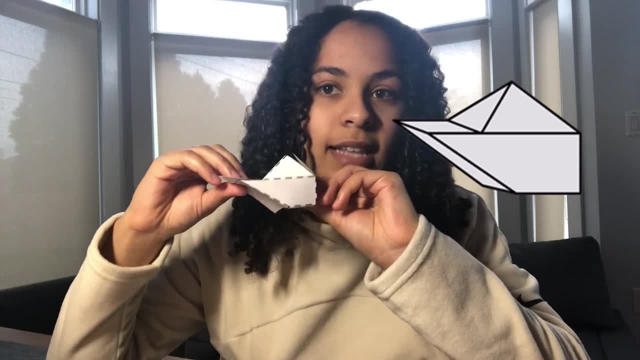 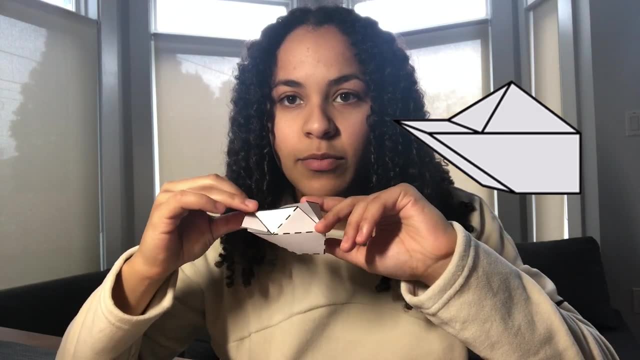 Right, And then you have that little like slant here. The square is the bottom And this rectangle on the top which covers this little piece, And this should be folded over, but I can't get it to stay, So yeah. 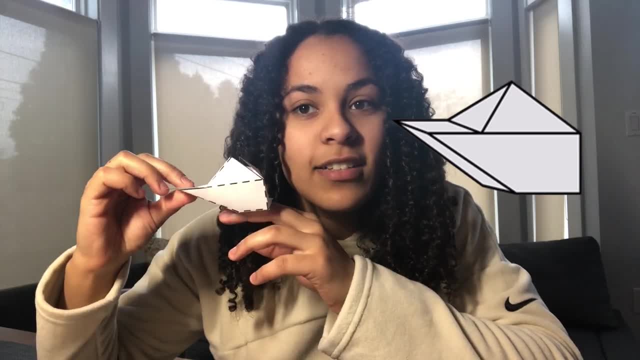 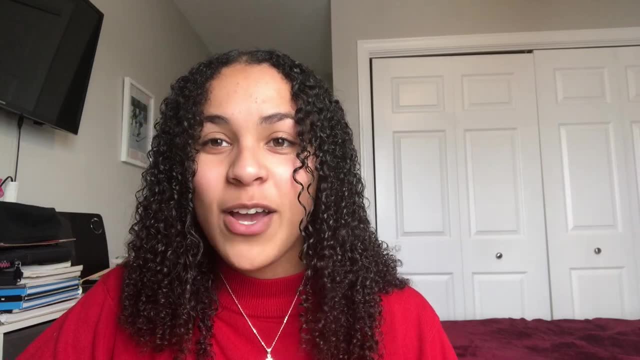 That proves to you that that is, in fact, the correct answer. All right guys. So I hope you enjoyed that video. I hope you got some value from it. Spatial ability is a bit tricky. It's a bit fast. Just you know pace yourself. 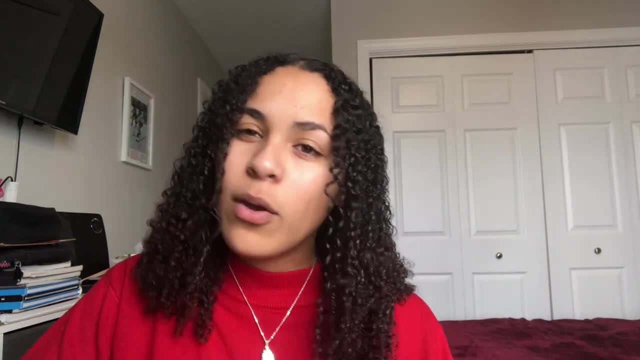 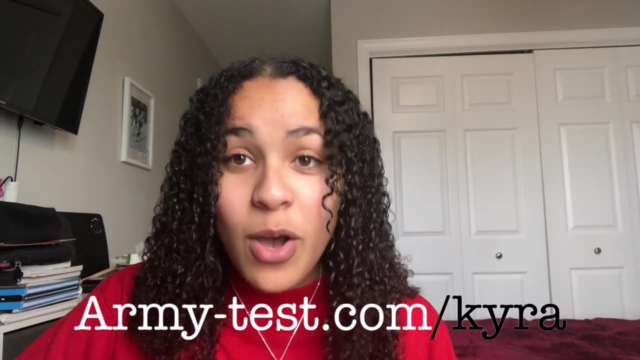 Keep an eye on the clock, Maybe find a way that works for you to think about these problems and just practice. If you need a lot to practice, like I said, armytestcom, You guys already know You can definitely get practice from there. 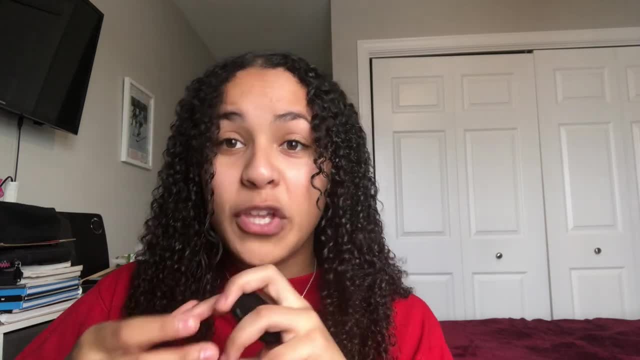 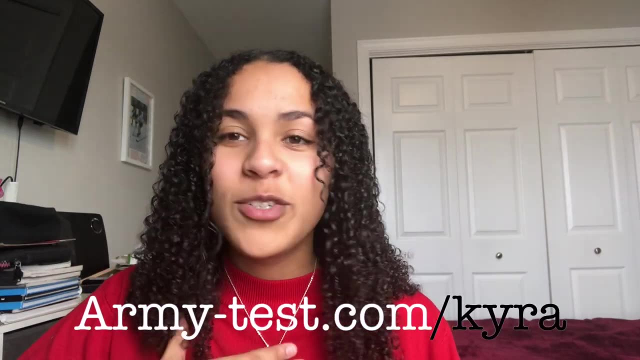 They also have like animations that fold up the cubes for you on a lot of their questions, So that really helps you think about it. You are going to sign up with that program. Please use my link, which is army-testcom. forward slash Kyra, which is K-Y-R-A.